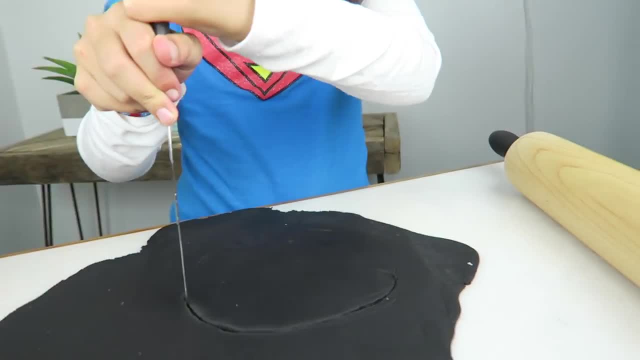 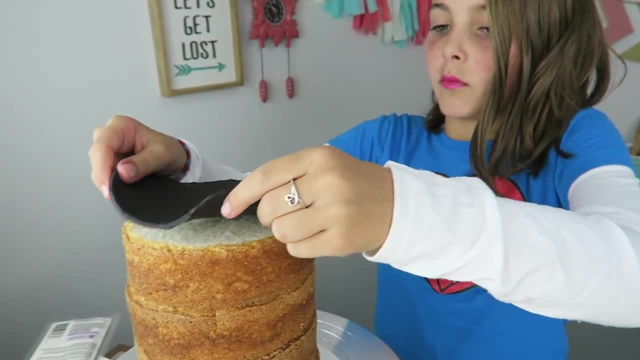 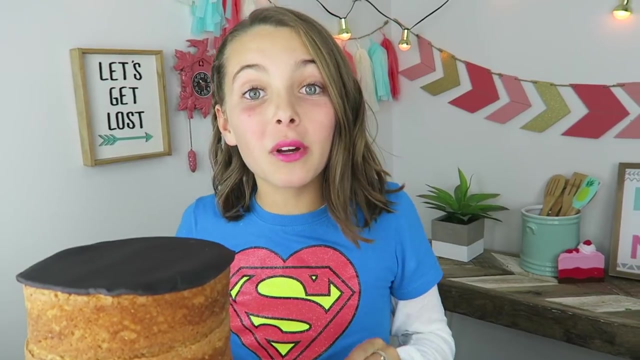 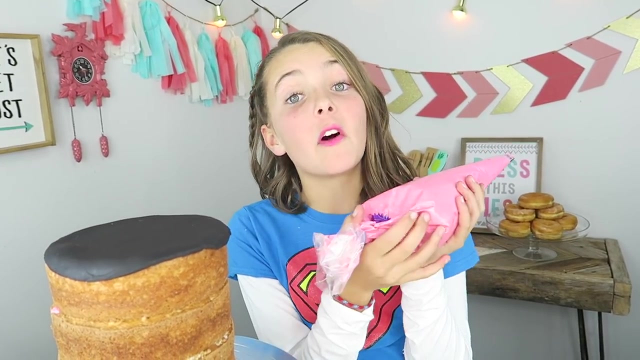 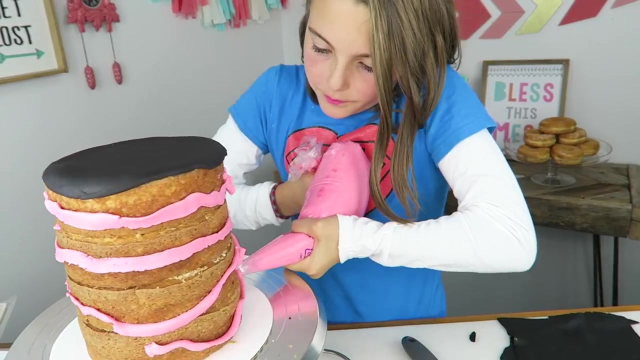 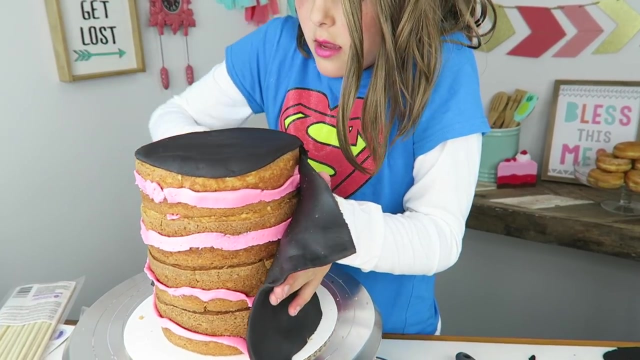 around the cake. Now we've got to cover the sides. This time I'm going to cut out a rectangle. Before we put the black fondant rectangle on, we've got to put a layer of frosting- Carefulcareful. It's like wrapping a baby in a blanket. 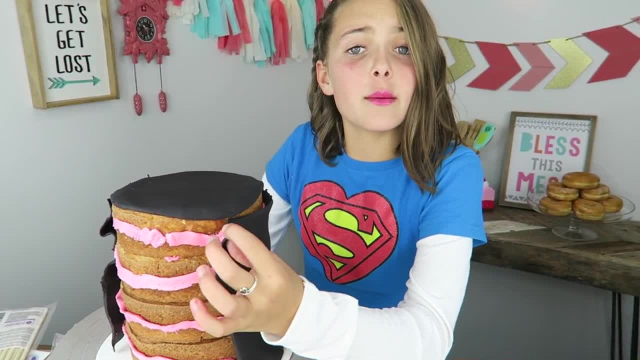 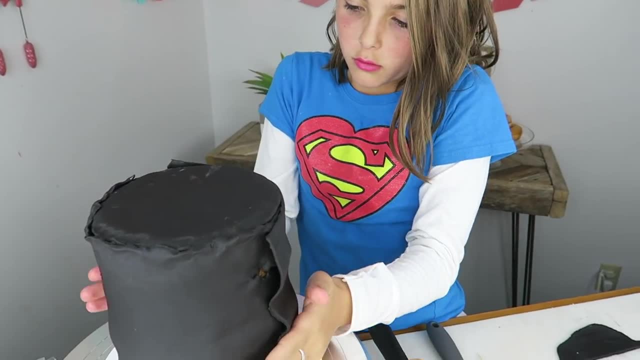 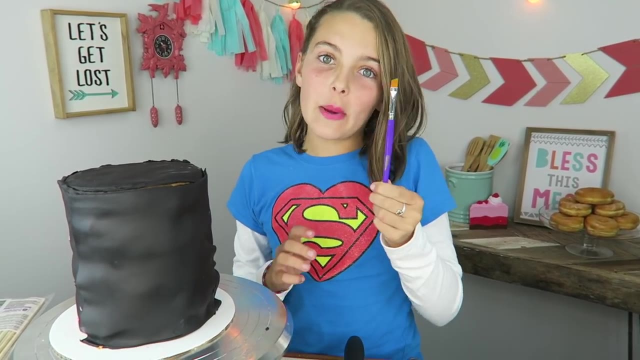 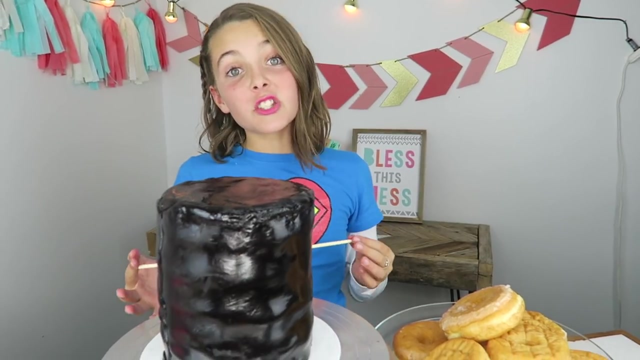 A little bit of frosting. Okay, It's starting to look like our tube of lipstick. I'm going to smooth it out with some water and a paint brush. Okay, we just finished the tube of our lipstick. Now we're going to add our donut part. 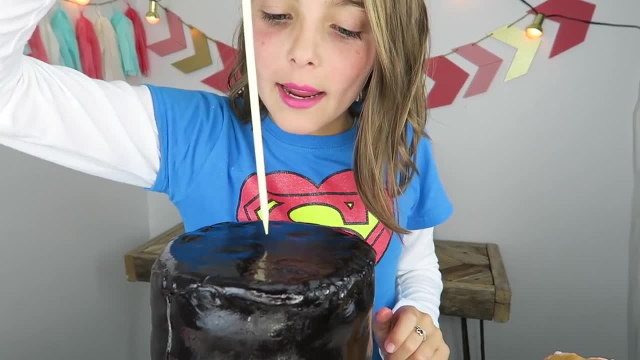 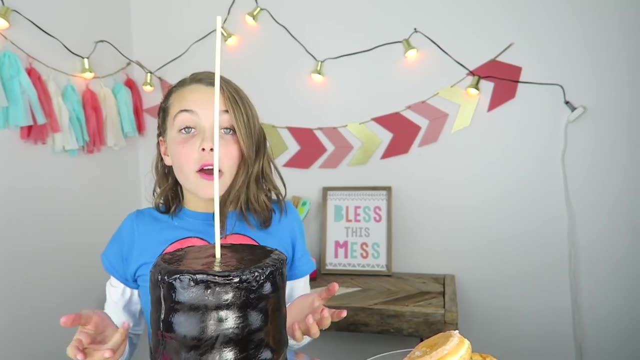 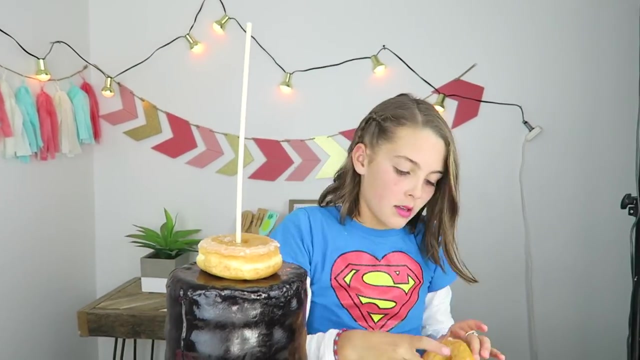 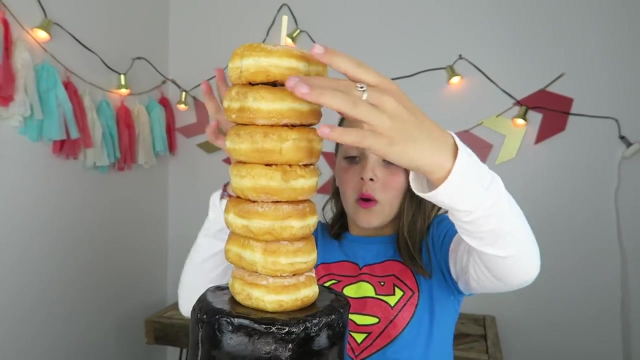 I'm going to grab this kebab stick and stick it right in the center. Only about this far. Now I'm going to put all of my donuts on it, So like this one. Whoa, this is going to be a tall cake. 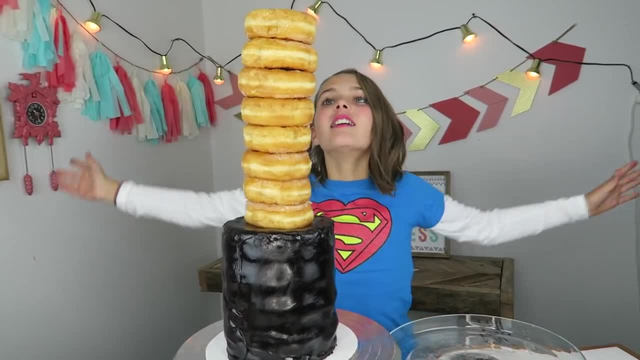 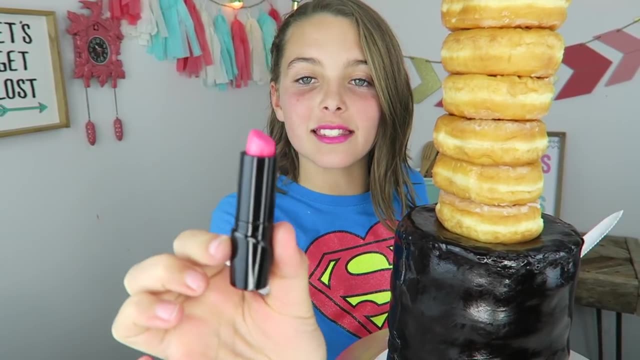 Last one: Ta da Peek a boo. I'm going to put this on top of my donut, Okay, So now we're going to take off the top donut and cut it into a slant. See how the lipstick is in a slant. 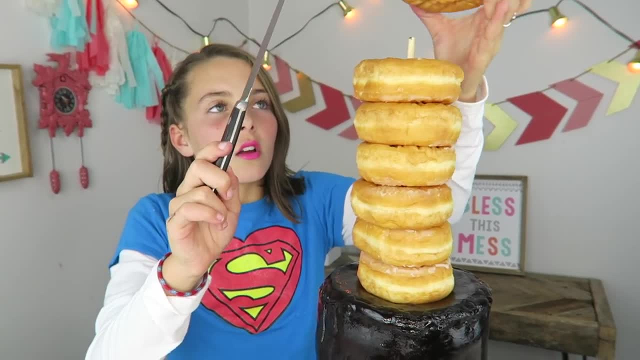 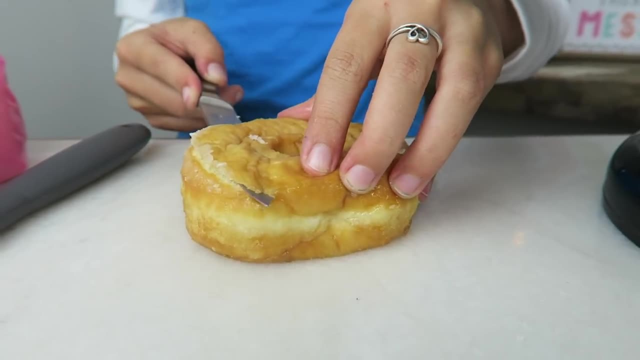 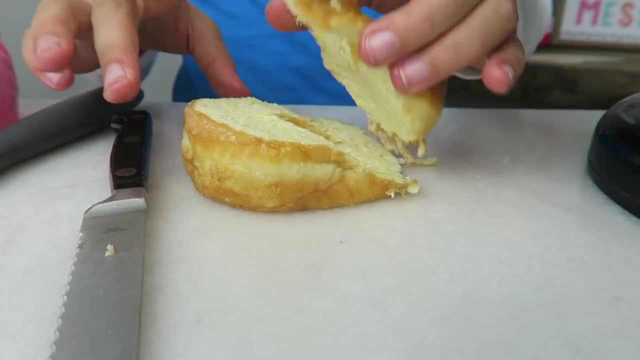 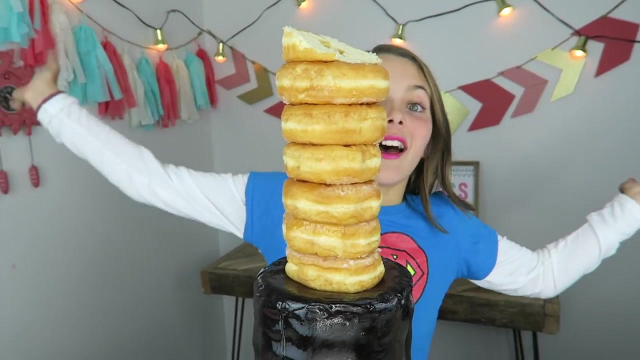 It's kind of like this Slant. Okay, So I just start at the top and then I keep on going and then I end up at the bottom on the other side, And then we put it back on. Okay, Ta da. 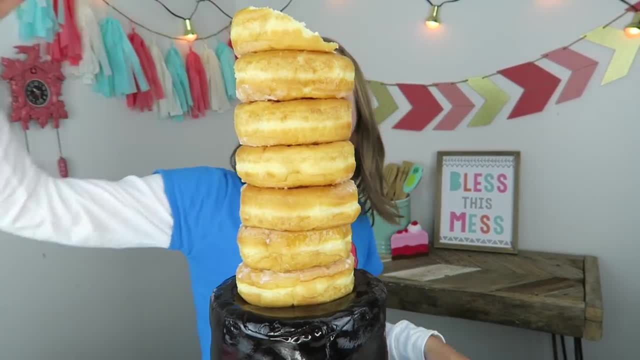 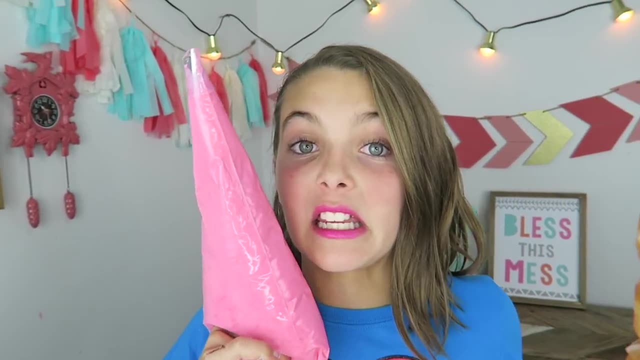 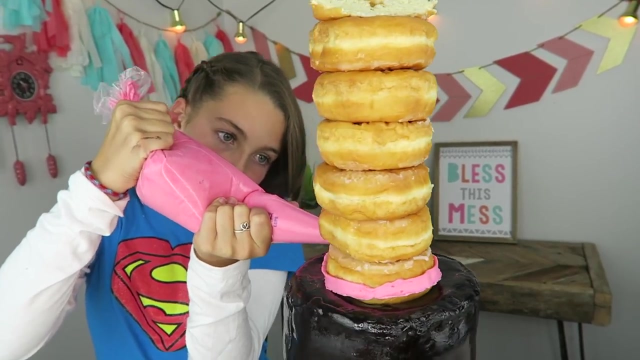 See how it's slanted. It's like downhill. It's a water slide. Wee Time for some more frosting. The pink matches my lipstick. I'm going to start at the bottom and then work my way up. There we go. 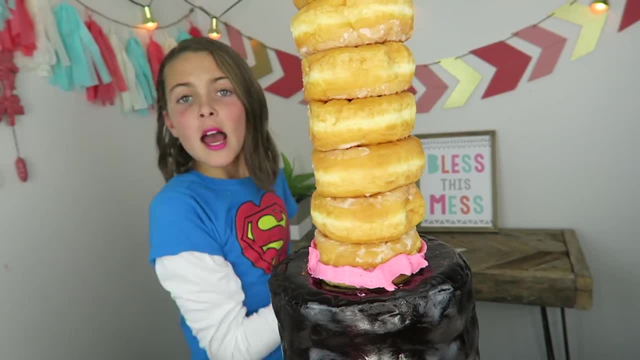 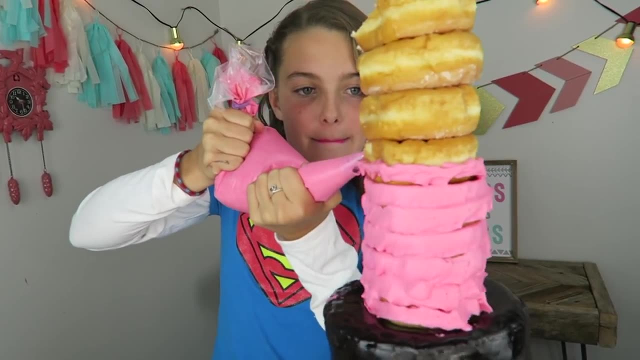 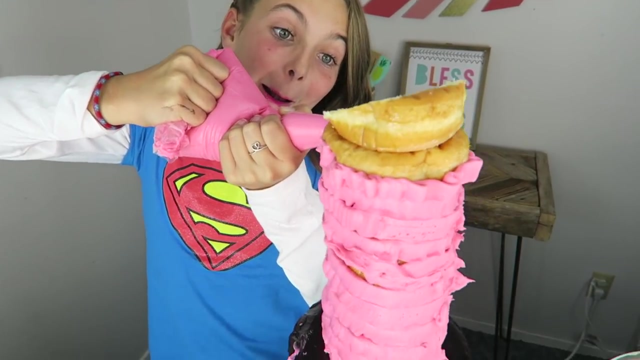 Woo Off to a pretty good start. Wait, I'm going to fill in this cream, Okay, Okay, Okay, Oh, that's not going to work. Nope, Whoopsies, We're almost done. It's like taller than me. 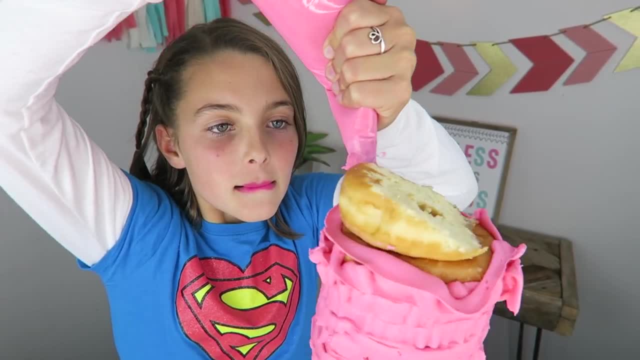 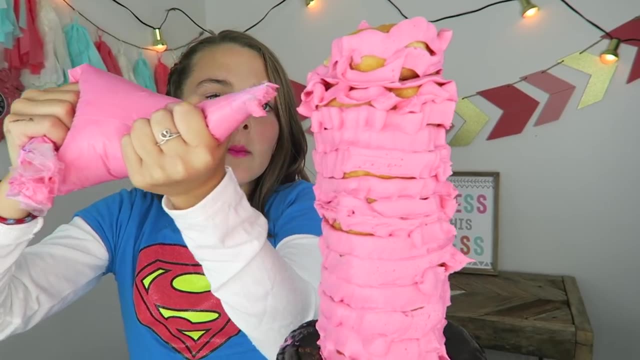 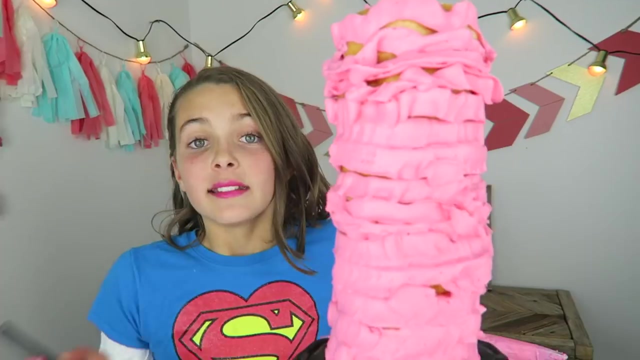 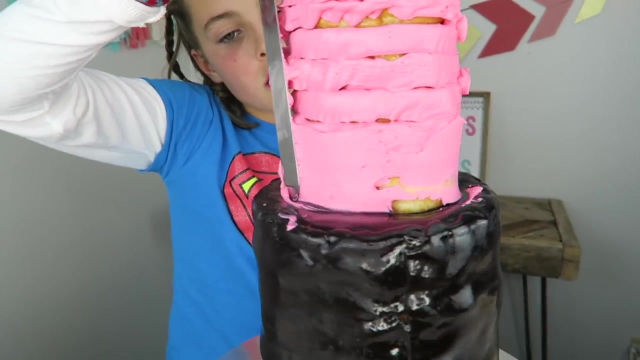 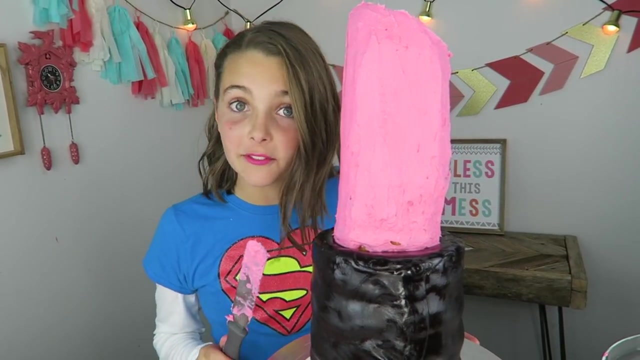 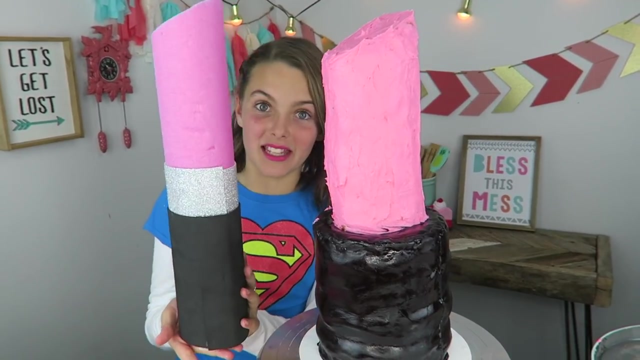 I need to get a stool. Okay, Okay, There, There. now we gotta smooth it out. If you have a friend that loves makeup, this would be a great birthday cake for them. Do you know what this reminds me of Our giant lipstick? 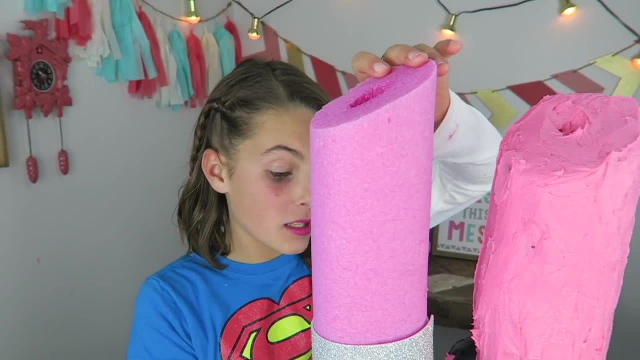 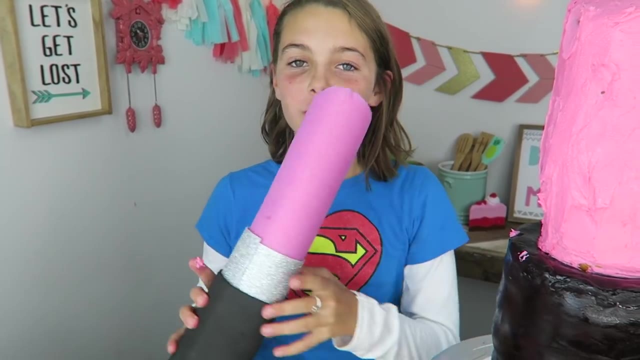 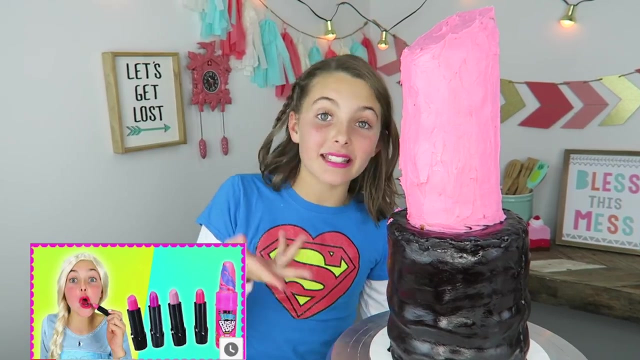 Like. this is like the exact same size. That is amazing. If you guys haven't seen this video yet, you guys have to see it. We made it out of a pool noodle, Anyway. Also, if you haven't seen our candy lipstick video. 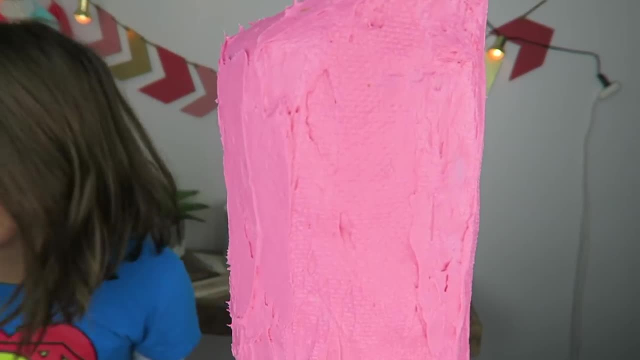 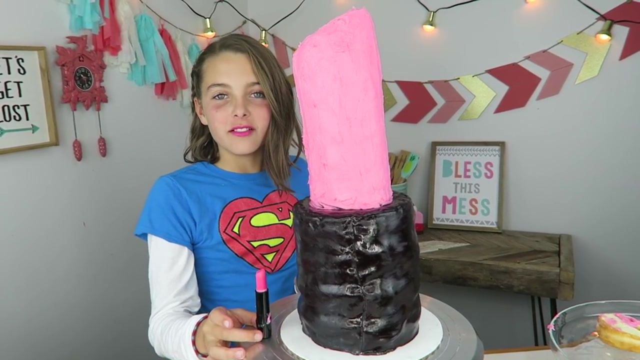 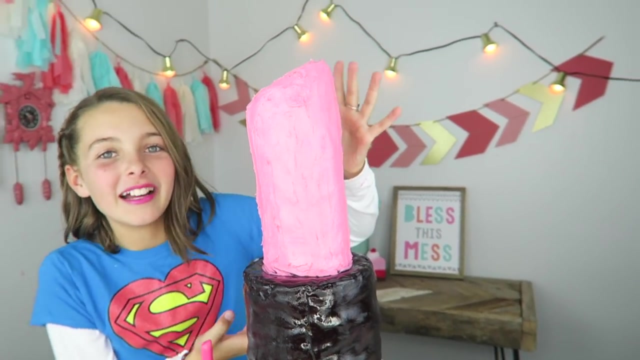 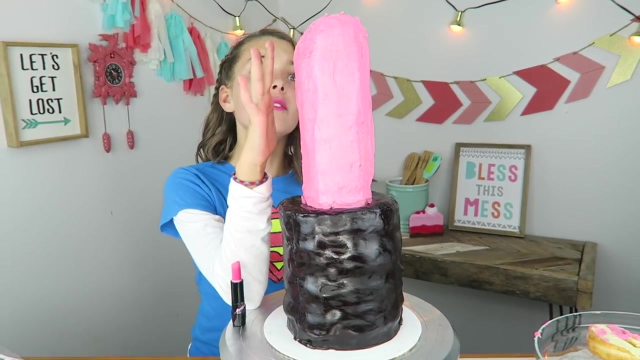 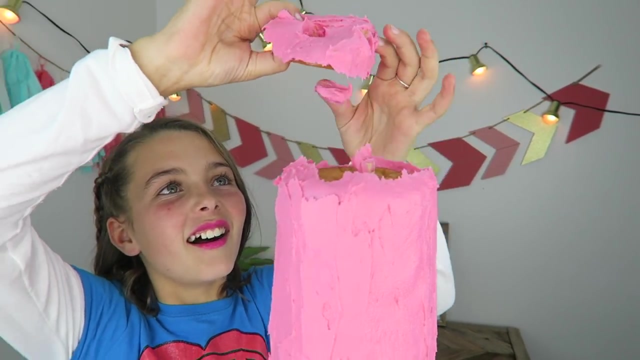 you should watch that one too. Which one is better? Which one would you use, Number one or number two? It's ginormous. It's like as big as my arm. That is cool. Time for a taste test Ready. 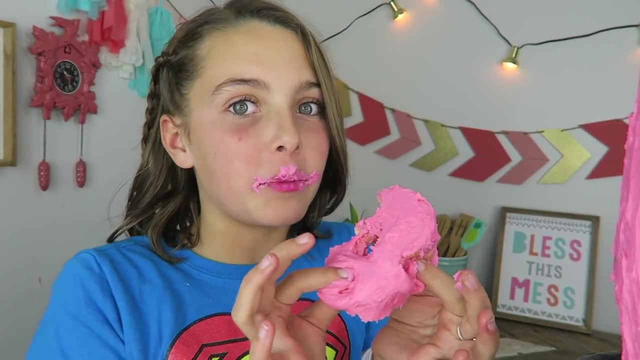 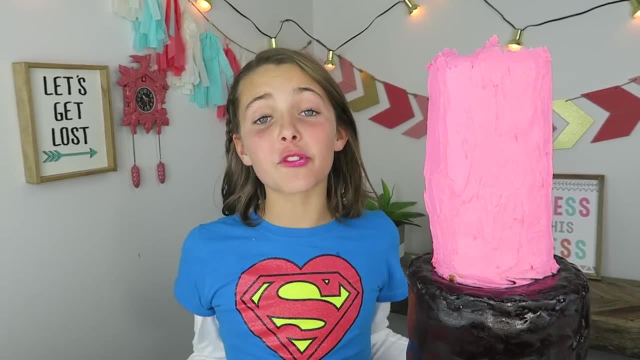 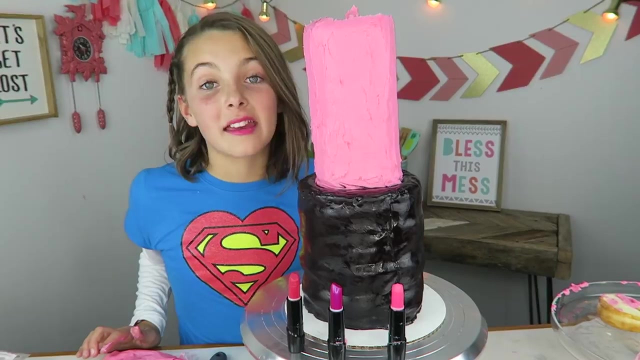 That's good. You can have a little snack and put your lipstick on at the same time. Thank you, guys, so much for joining me today. Don't forget to like, subscribe and comment down below. Comment down below. And comment down below. what shade of lipstick? 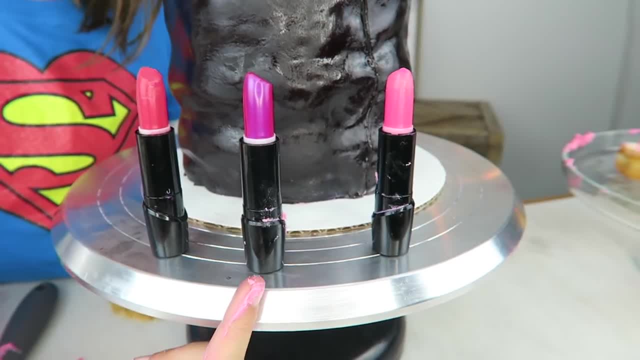 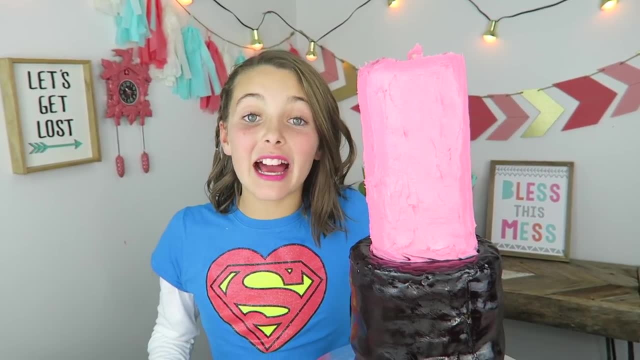 is your favorite? Number one, number two or number three Or number four? Have a great day, guys. See you later, Bye, Bye.